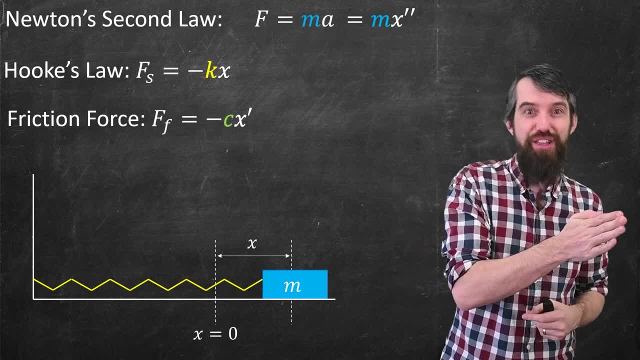 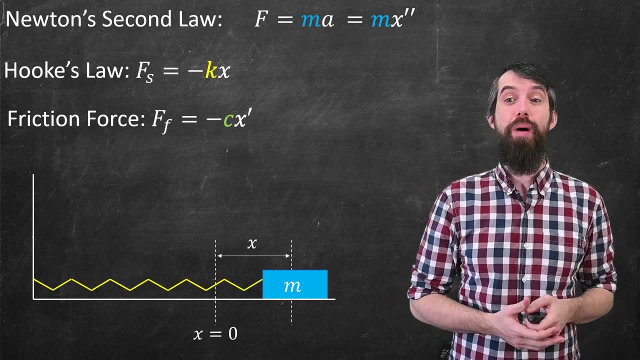 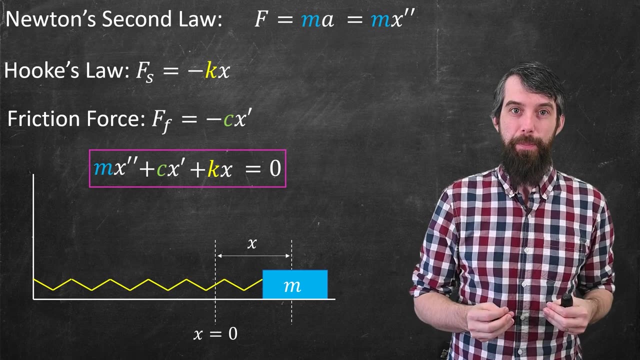 force pushes against the direction in which you're traveling. If you're traveling this way, the force is an impediment to your motion Either way, since Newton's law is the sum of the forces, I can combine all of these things and say that mx double prime plus cx, prime plus kx is equal to zero, And 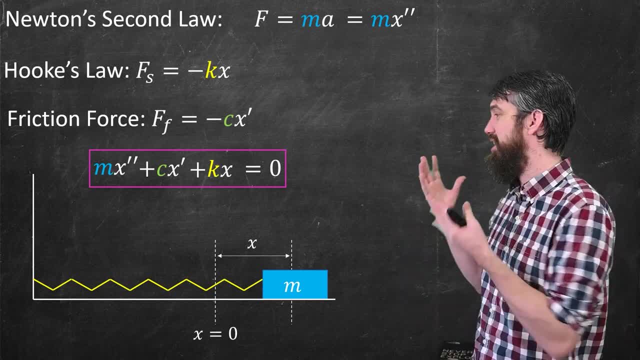 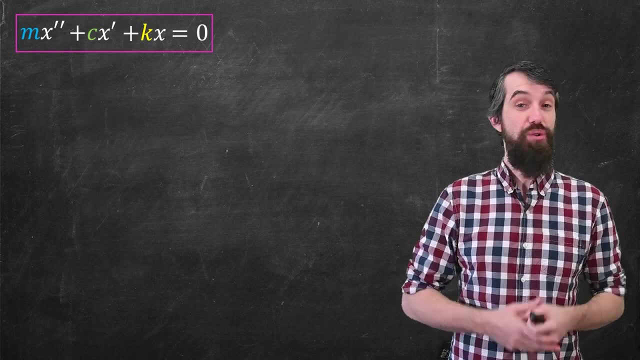 now what I have is a different force, And if you're driving at a speed of x prime, you're going to have a differential equation. I can forget the context. This is just a second order constant coefficient differential equation, So let's try and solve it. Okay. so what I'm going to do is the. 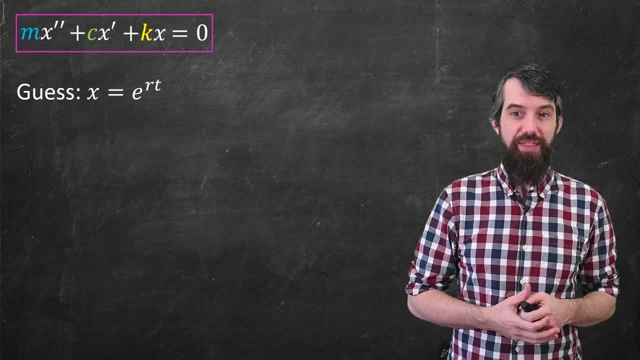 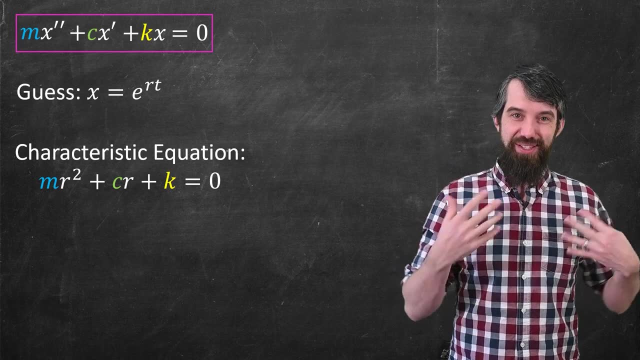 same trick I always do. I'm going to guess x is equal to e to the rt. I plug this in. I get a characteristic equation of mr squared: plus cr plus k is equal to zero, as well as an e to the rt on. 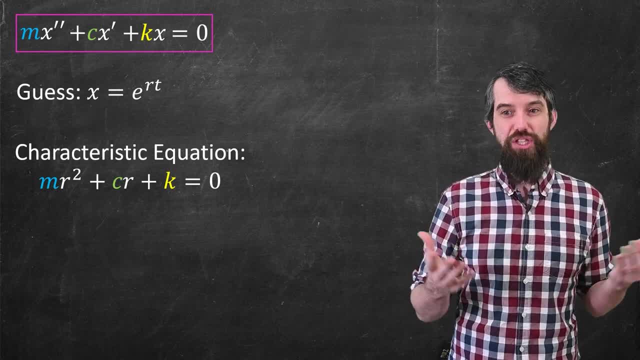 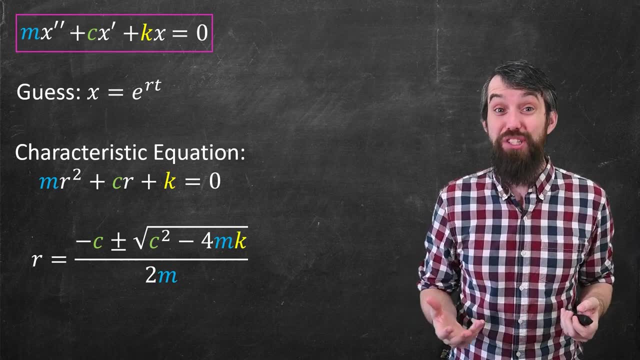 every term, which I would cancel. And then, if I want to solve for my r, well, it's just the quadratic formula here. Okay, so now there's a quadratic formula, but I've got these arbitrary constants, And so there's actually a bunch of different cases of what this quadratic formula. 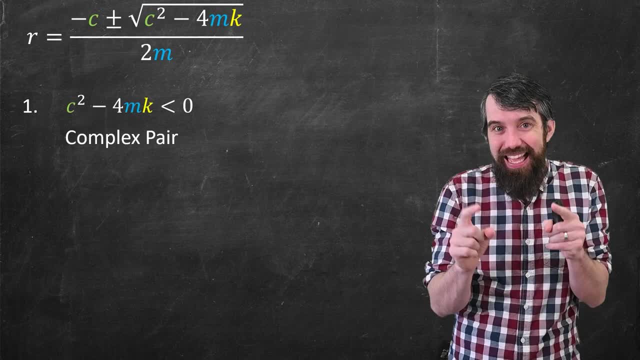 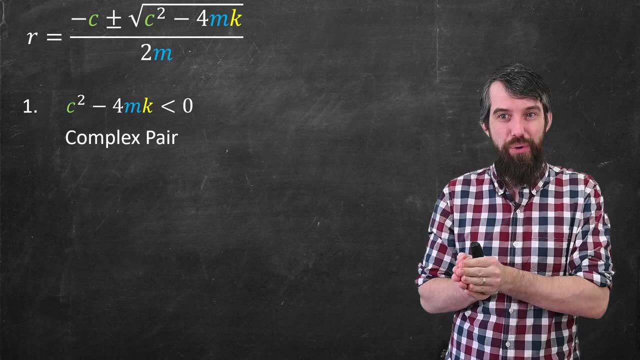 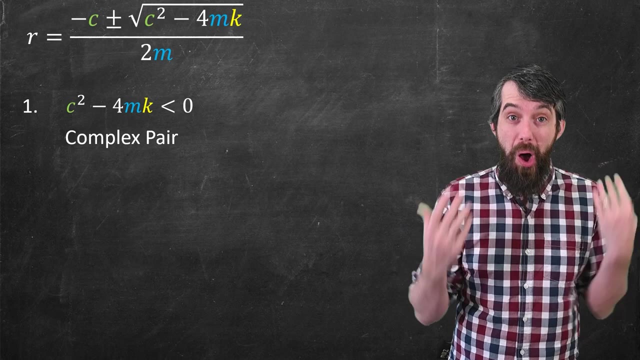 could do. Case one could be that the thing under the square root is negative- It's less than zero- in which case you'd have a complex pair of roots. The square root of a negative would be imaginary. The other case would be that the thing underneath the square root would be positive, in which case 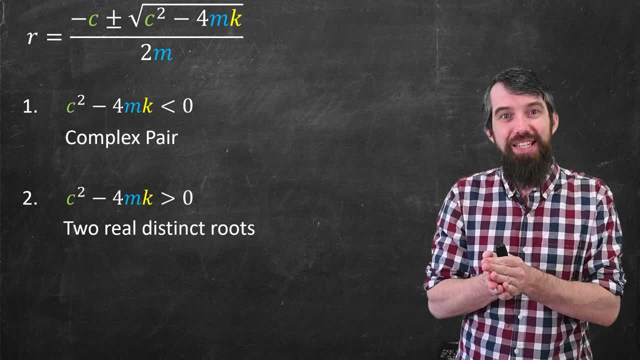 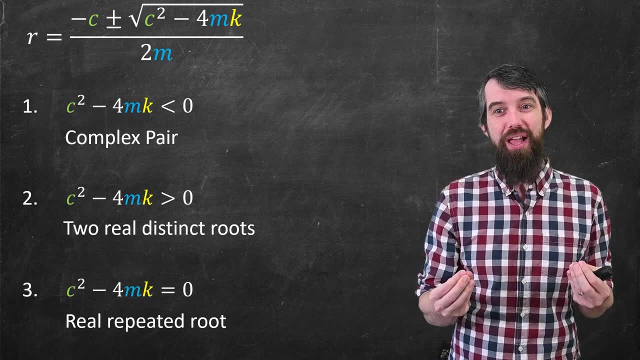 you'd have minus c over 2m, plus something and minus something real. You'd get two real and negative roots. And the third case would be that the thing under the square root was zero, in which case you'd get plus or minus zero. You'd just get the same root with multiplicity 2. We call that a. 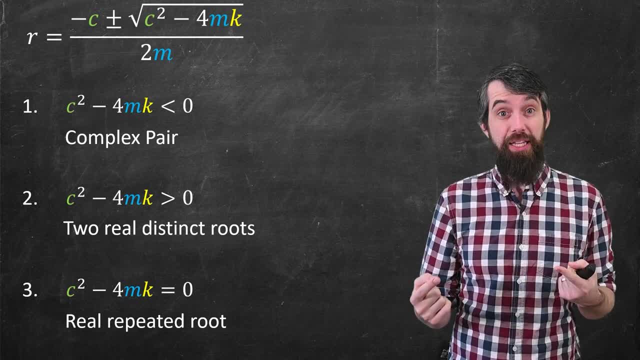 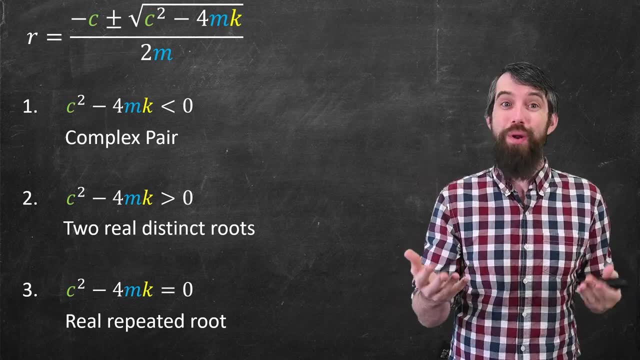 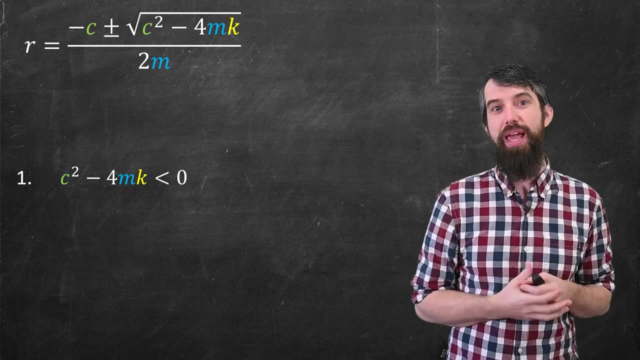 real repeated root. So we've seen these possibilities when we've studied constant coefficient equations before. but what I want to do is interpret each of these three things physically. What does that mean physically in the context of a mass on a spring? So let's deal with the complex case first. where c squared minus 4mk is negative, This is called 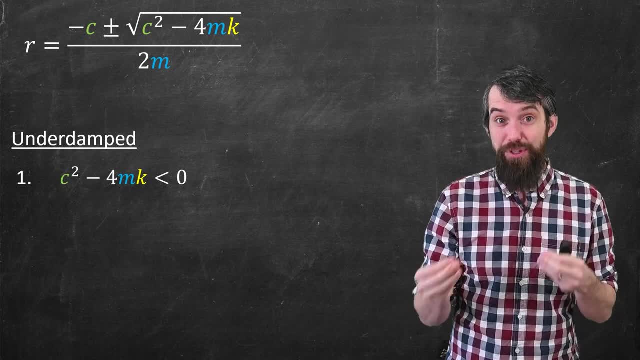 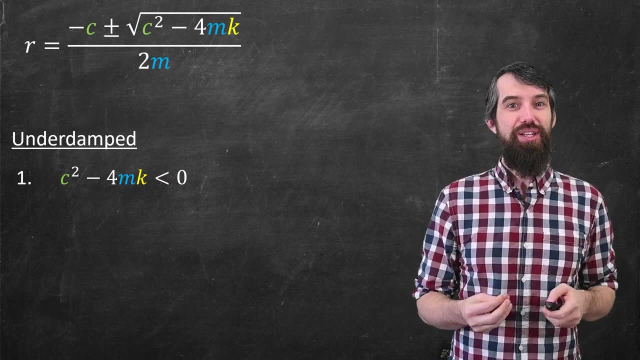 the underdamped case, That is, the damping which comes from the c value, is smaller, and this makes this thing negative. So what I actually really want to do is take the roots r and break them up into the real and complex part, So I'm going to separate it. I've got a minus c over 2m on the. 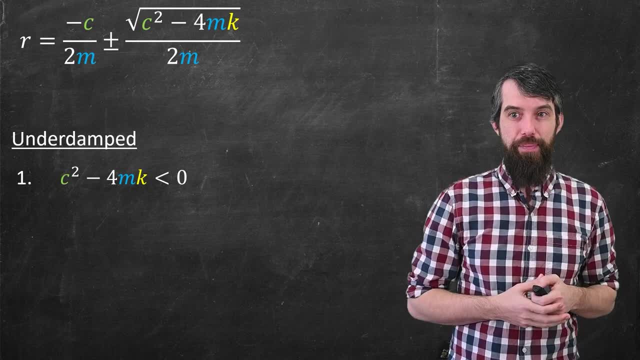 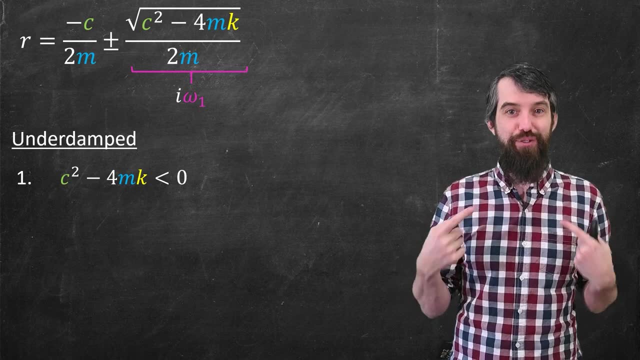 left. That's real, And then plus or minus something imaginary, And I'm actually going to relabel it. I'm just going to call this i omega 1 here, So square root of c squared minus 4mk all divided by 2m. That whole thing is going to be imaginary. I'm going to call this i omega 1 here, So square root of c squared minus 4mk, all divided by 2m. That whole thing is going to be. 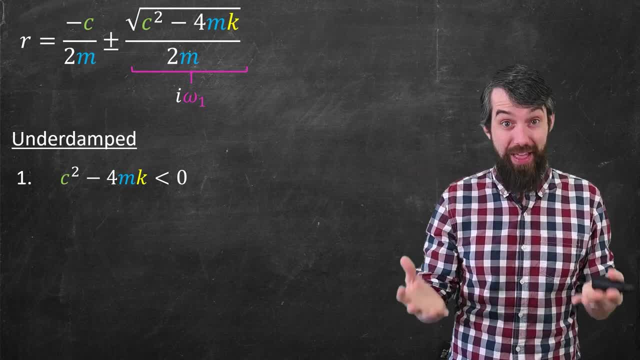 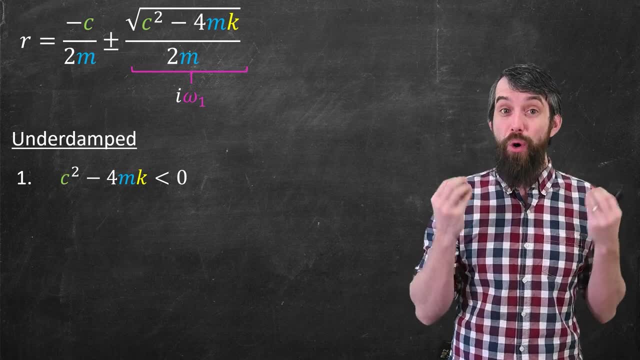 imaginary. It's an imaginary number times omega 1.. That's my definition. Now, in the previous video we talked about mechanical vibrations with no friction. We had something called omega naught, And omega naught was just square root of k over m. But if you went to this formula, 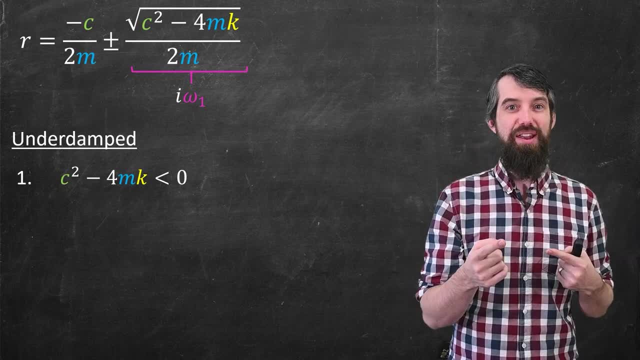 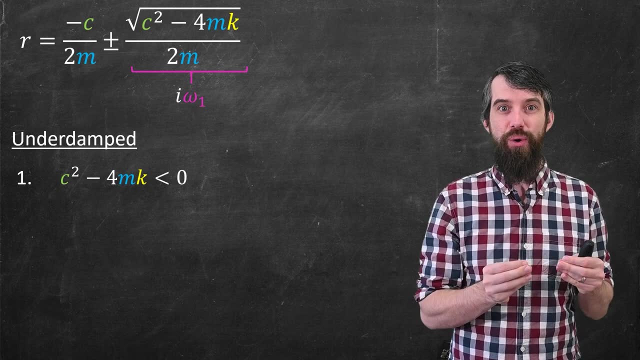 you plugged in c equal to zero, the fours would cancel and you'd have a square root m on the top and an m on the bottom. That would become square root of k over m as well. So in the case where c equal to zero, omega 1 is just equal to omega naught. 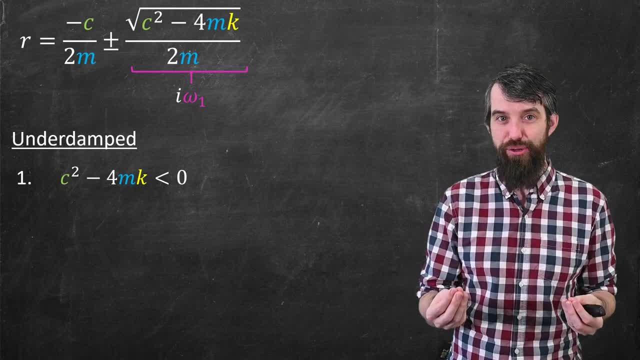 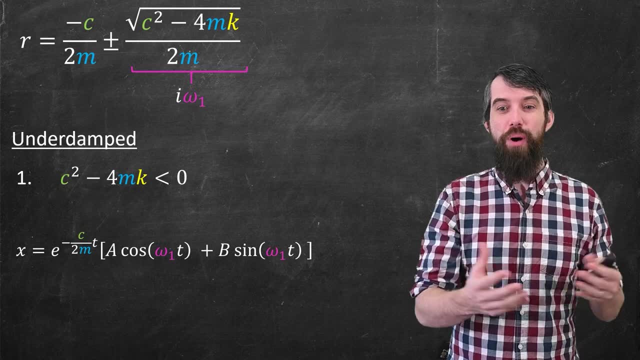 Okay, so that's fine. And now we can state what the solution is: knowing how to solve constant coefficients. That is, our general solution is well, e to the real component times t. So e to the negative, c over 2m times t, And then the contribution of the imaginary parts. 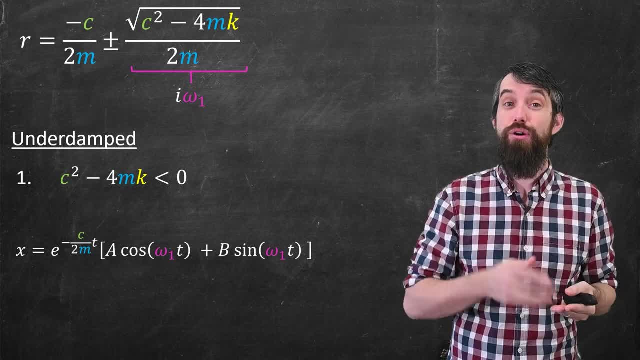 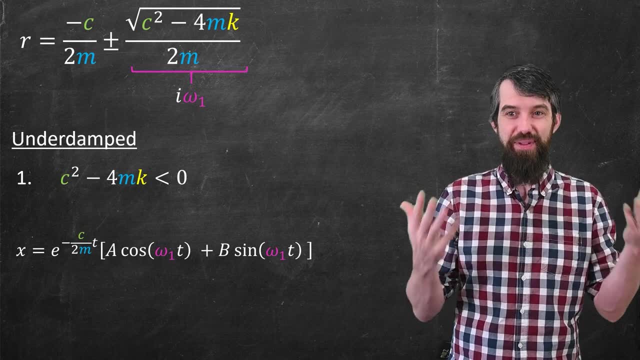 is going to be a cosine term and a sine term, So a cos omega 1 times t and b sine omega 1 times t. It's just convenient to have these frequencies omega 1 in here. It's going to make this just all. 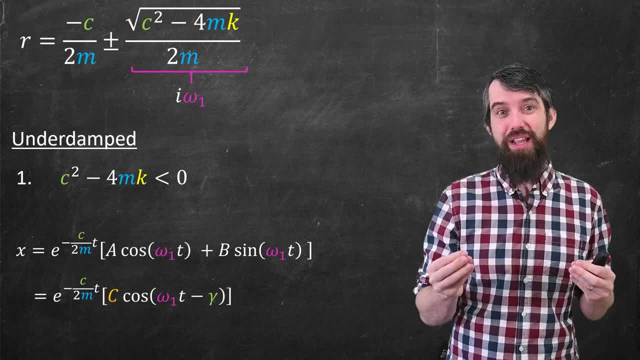 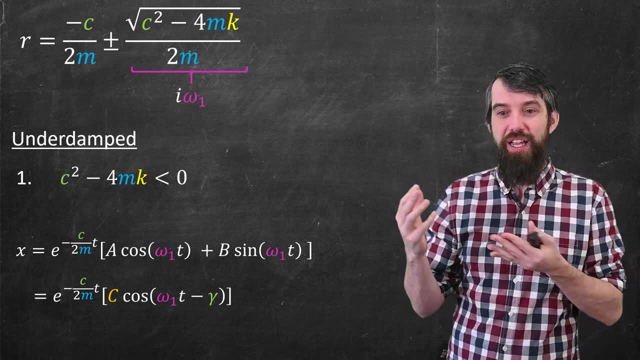 a little bit shorter to write down Now, I can still do the same trick that we did in the previous video. in the frictionless case, As in, I have a cosine and a sine term and I can do this shift. that makes it just become: 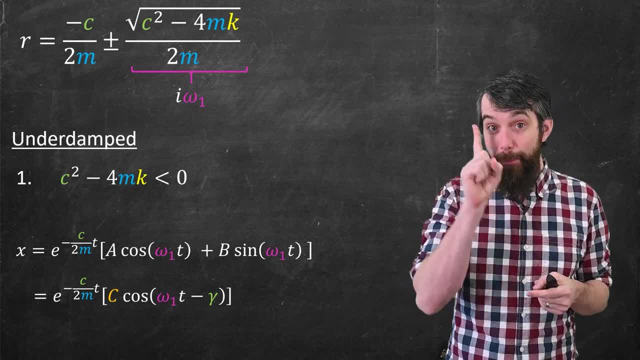 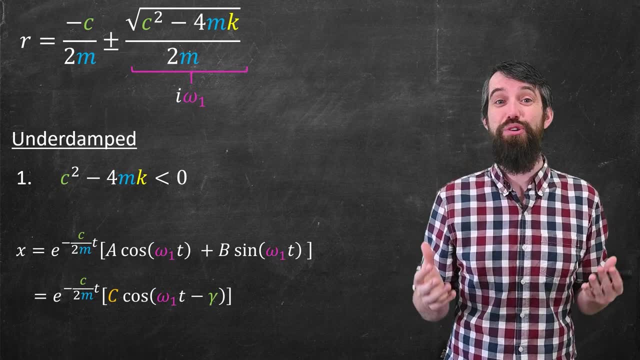 a single cosine, term c: cosine of omega 1, t minus gamma, that little offset, And we'll talk about exactly what that's going to mean in a moment. Okay, so let's try to get a sense of what's going on here graphically. So now I'm going to grab this. What I've inputted in is a constant times. 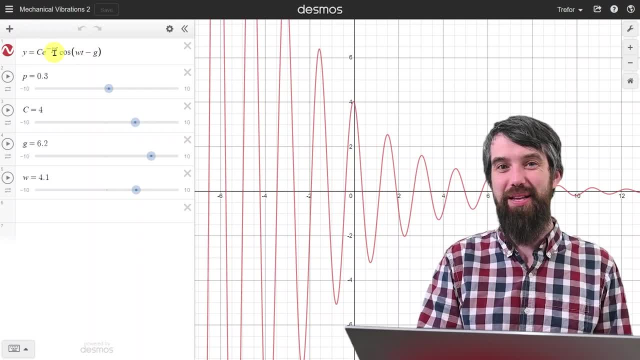 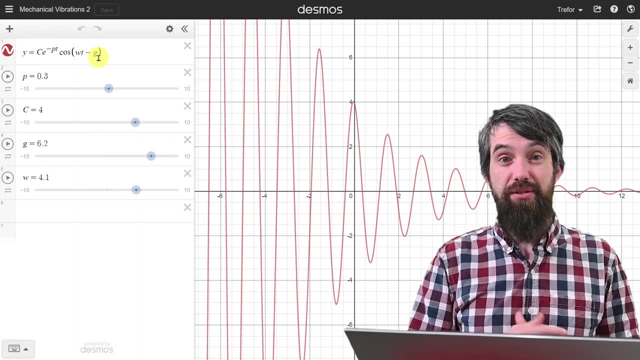 the negative exponential. I just call that e to the minus 1t. So I'm going to write down the p, where p is some positive number, And then cosine of what we could call omega 1, t, and then minus the shift, gamma or g using Roman characters. So what's going on here? Well, the c, the g, 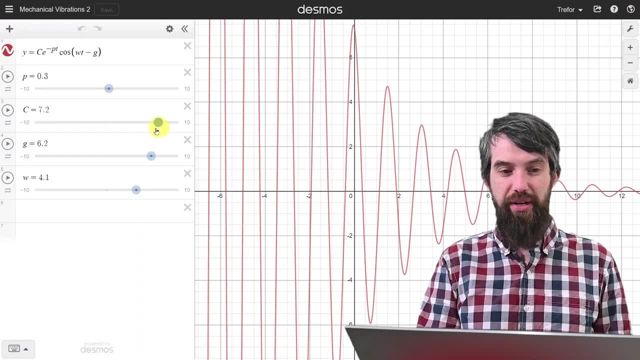 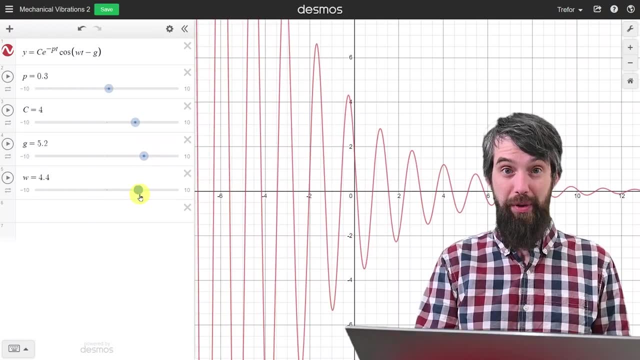 and the w. we've played with them before. If you increase the c, you increase the amplitude. If you increase the g, you just shift everything left and right, And if you change the omega, you change the frequency. We've seen all of those before in the frictionless case. What's new here is the value of 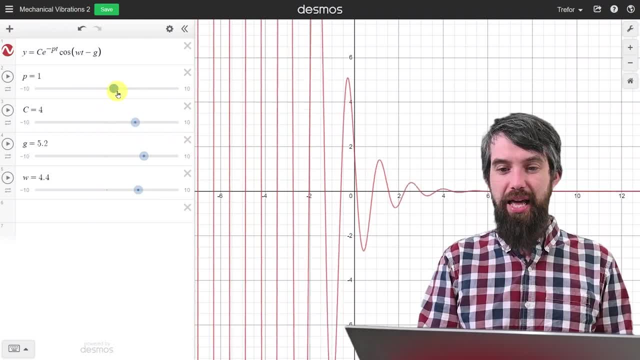 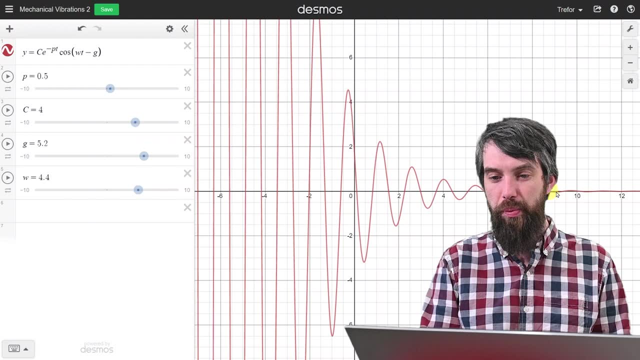 this p, And what we're going to do here is we're going to take the value of this p, and what we're going to notice by this exponential growth is that, as I increase it or decrease it, it changes the nature of what I'll call this envelope curve, Indeed, this top curve here, where I'm sort of 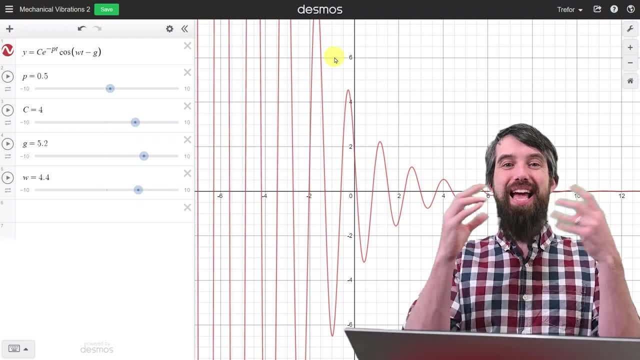 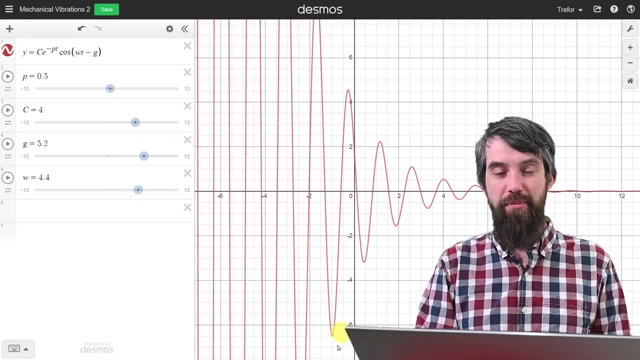 tracing along with my mouse here would just be the exponential without any trigonometric terms, without any oscillations. Likewise, this curve, that sort of envelopes along the bottom, would be the negative of that exponential without any sine or cos terms. So you can sort of imagine having 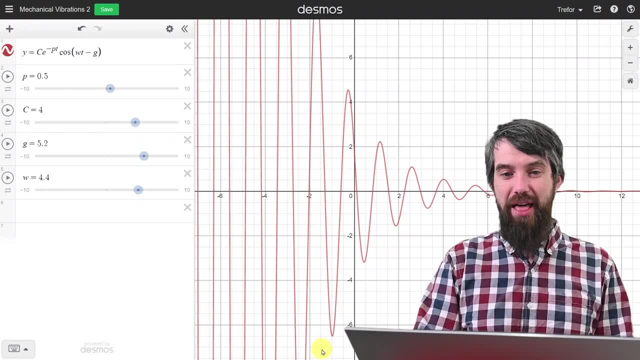 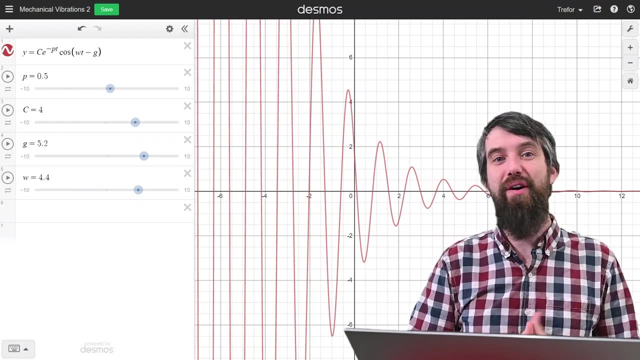 this envelope here of the e to the minus 1t, And what I'm going to do here is I'm going to take the exponential and its negative and then what happens is the curve oscillates back and forth in between that And so as t goes to infinity because it's a negative in the exponent of our 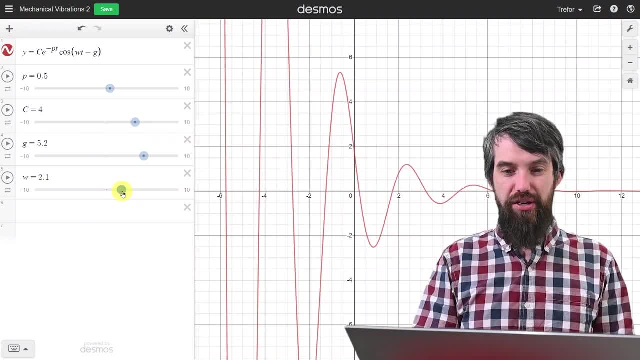 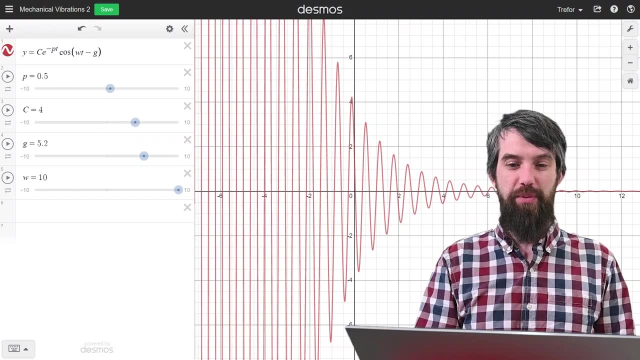 exponential, it just drops it down to zero. And you can sort of see, if I take the frequency slider and drag it all the way to the right, that envelope curve becomes just a little bit more transparent. You might choose to ignore what happens before t equal to zero. If you plot this, 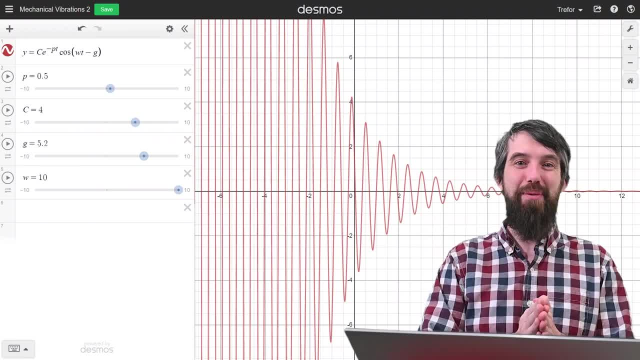 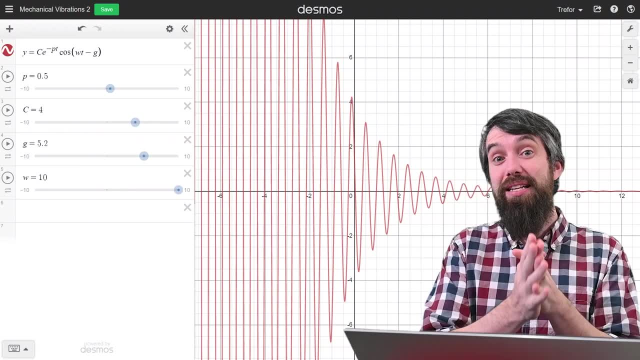 backward for negative t's. you can see that it's sort of blowing up, But maybe we'll imagine our only considering about t equal to zero. So what we're going to do here is we're going to plot the t greater than zero scenario in our model. Okay, and then, if I try to translate this: 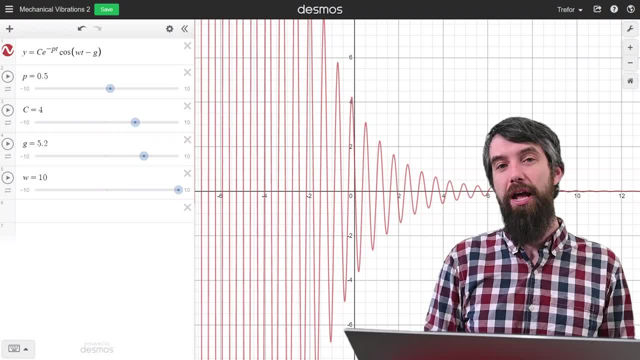 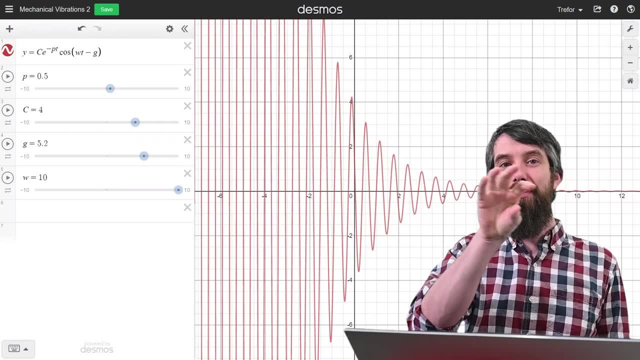 graph into the physical situation of my block going back and forth. the idea is that it oscillates back and forth but because of the friction, the amplitude starts to get smaller and smaller, and smaller and smaller, until it just settles at the equilibrium point. That's what this is showing. 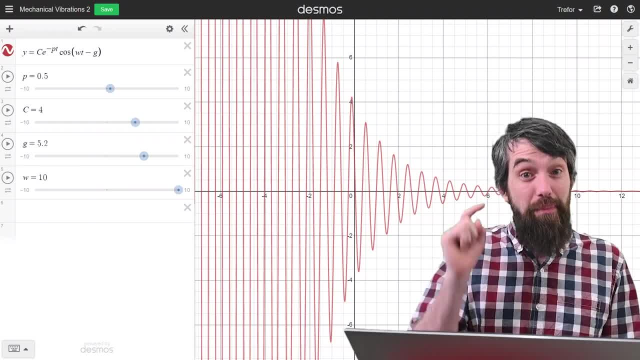 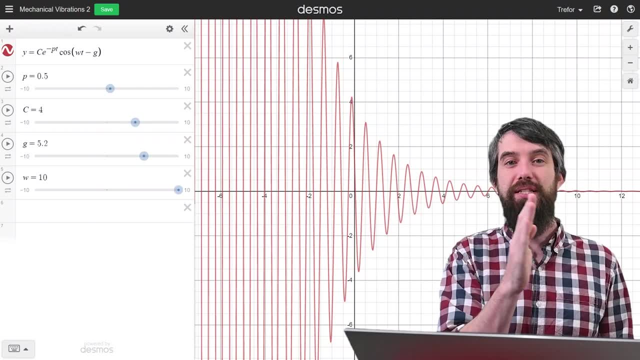 It's saying we still have the oscillations but that the amplitude is being diminished by the e to the negative pt. So it goes and has your oscillation back and forth, and then it's going back and forth but it lowers its amplitude And finally, as t goes to infinity, it's going to. 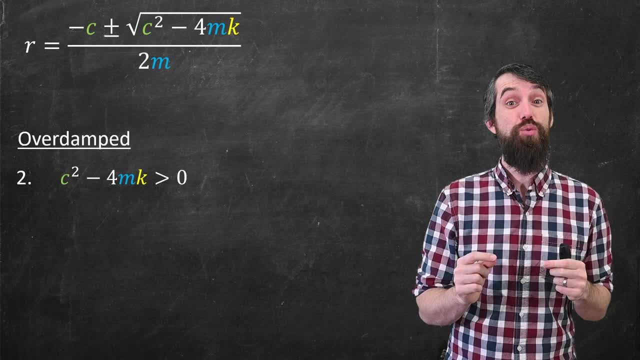 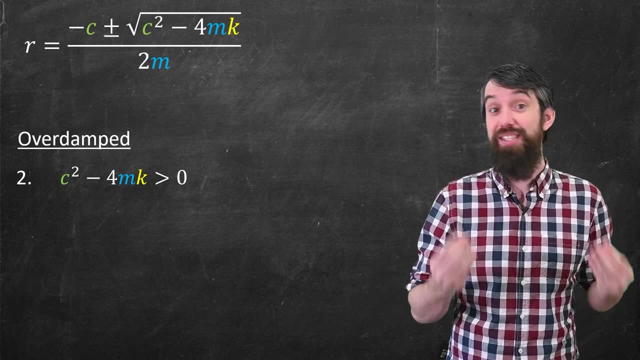 settle right down at that equilibrium point. The second case we're going to consider is what I call the overdamped case. So this is when c squared minus 4mk is greater than zero, when you have a lot of friction, So the c is a big number. Well, in that case we get these two different real. 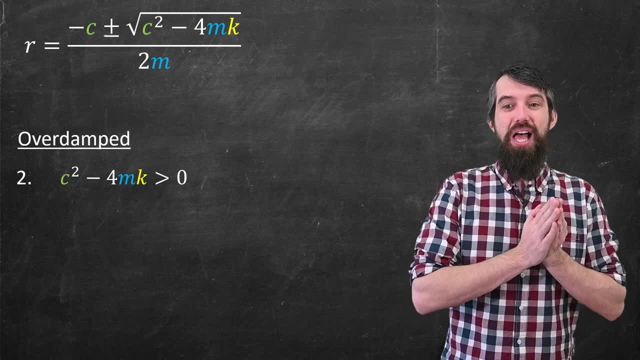 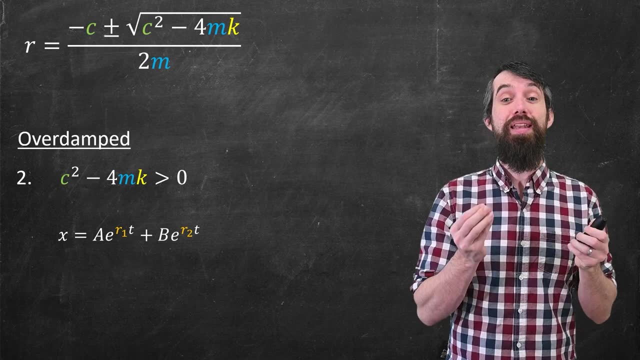 roots, And so what you're going to get is something to the form a times e to the r1t plus b times e to the r2t, where r1 and r2, those are both going to be negative values, So we're going to get a. 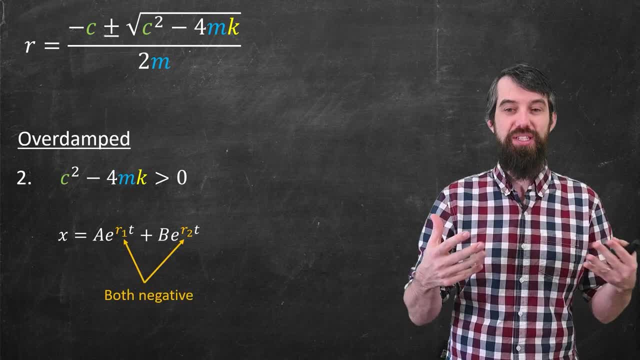 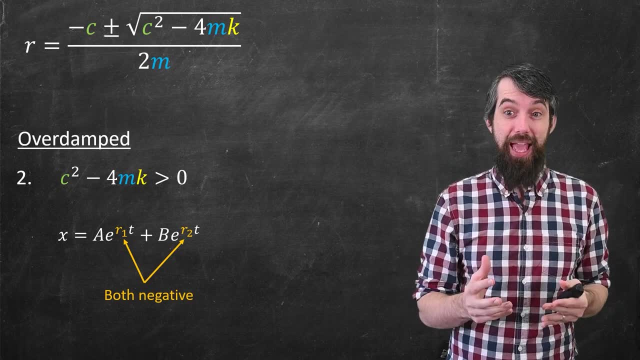 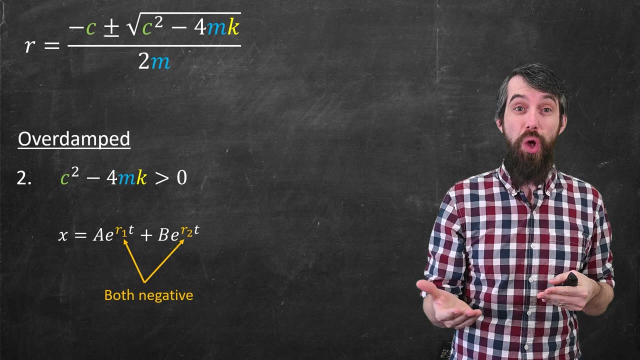 negative. So basically, as time goes on, x is going to go to zero. There's going to be an exponential decay. So what does this look like? Well, I don't even need to graph it to understand it, because they're both negative exponentials. As time goes on, it's just going to be exponential. 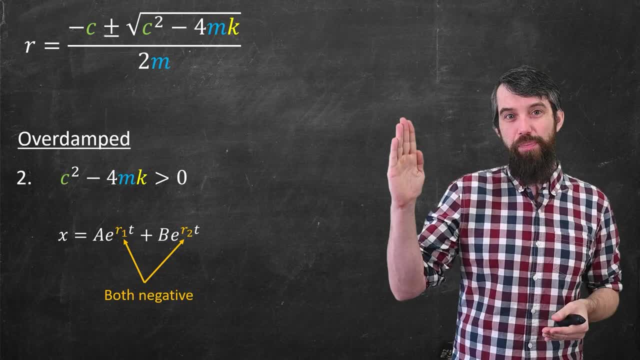 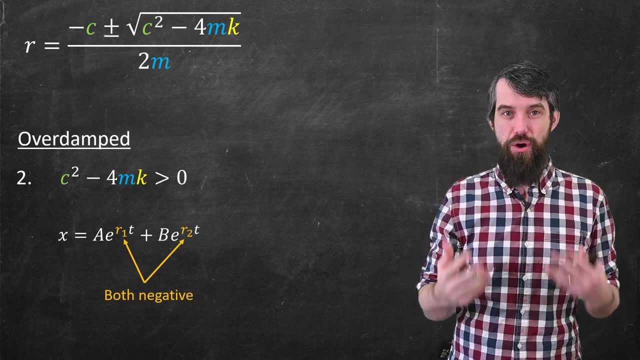 decay down to the value of x equal to zero. It's just going to be like a block that does this and settles on the equilibrium. So there's no oscillation here, right, There's no sine or cosine term, It's just this exponential decay back down to the equilibrium spot. 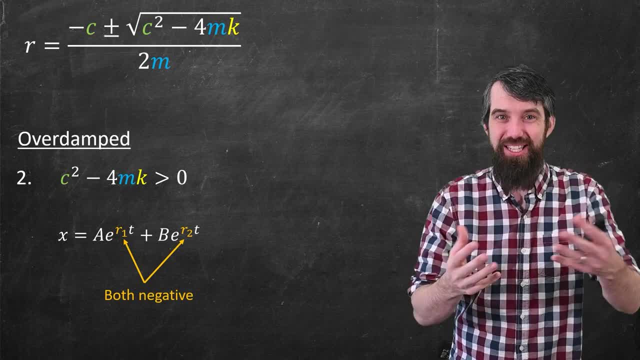 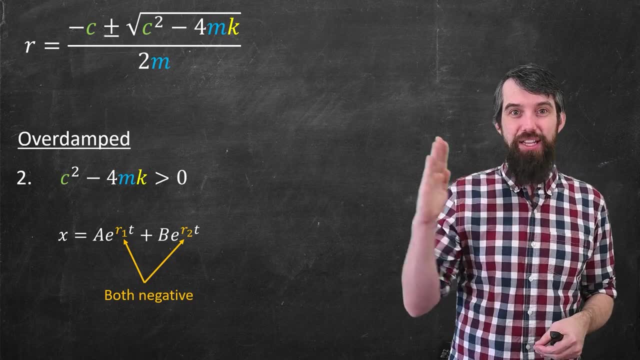 So the way I imagine this is like imagine your spring is in molasses or something- with this enormous amount of friction. It's so much friction that there actually isn't an allowed oscillation. It just starts off set from the equilibrium points and it decays down to the equilibrium point. 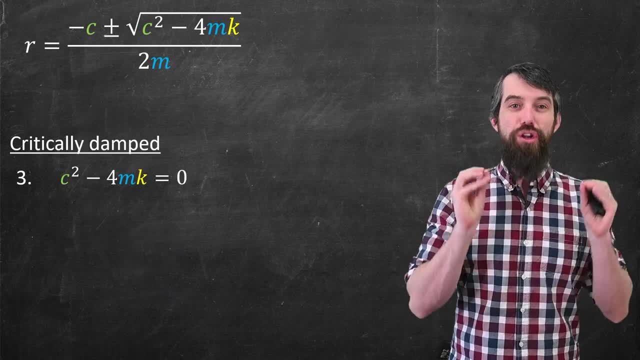 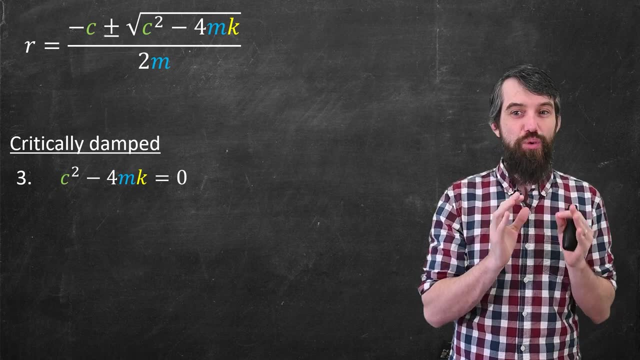 The third and final possibility is what is called critically damped. This is, of course, very rare. It's hard to have things being equal. It's hard to have things being equal to zero exactly, But this is when the c squared minus 4mk. 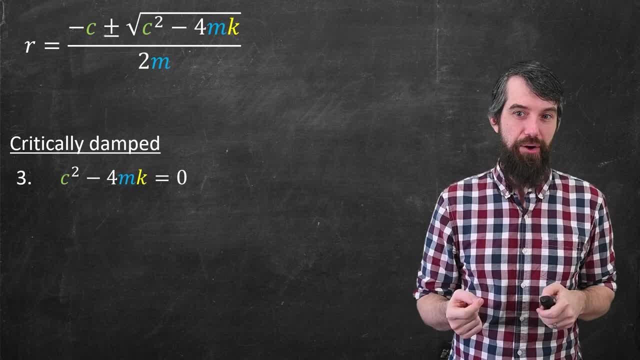 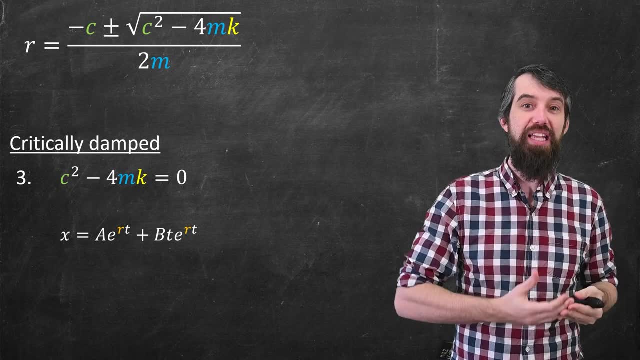 is precisely equal to zero. Now, what would happen in this scenario? Well, if you tried to solve it, we would say you've got repeated roots. and we knew that. the method for repeated roots is you take the one root e to the rt, But then for the second you can't just repeat it, because it would 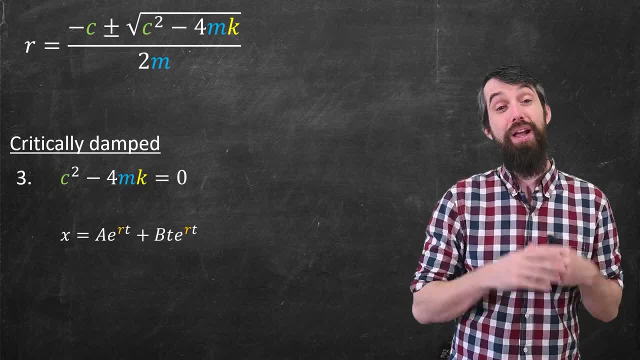 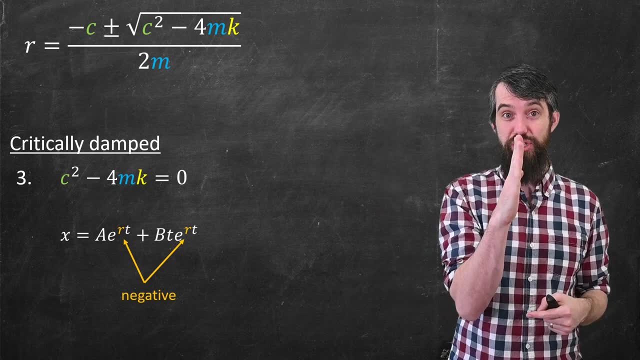 be e to the rt. again You do te to the rt. That's why it's b times t times e to the rt. The r is still negative, which makes it seem like it would just go right down with exponential decay back to the equilibrium point, kind of like in the overdamped case. But the t here. 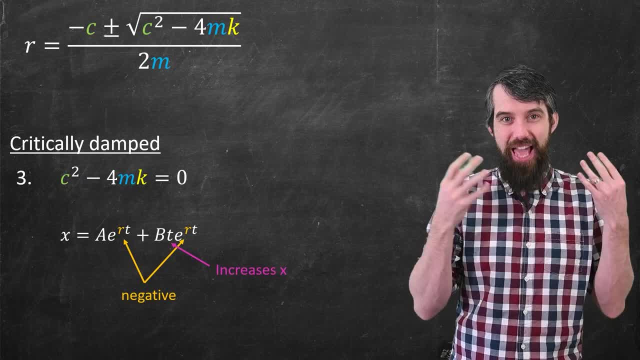 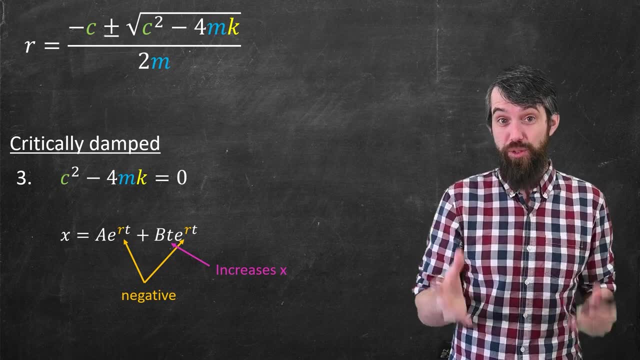 it means that it increases. So you have a sort of a competition of the facts. The exponential terms are dragging it down to zero, The t is making it larger. So let's just turn to the software to get a really good visual picture of what this one looks like. 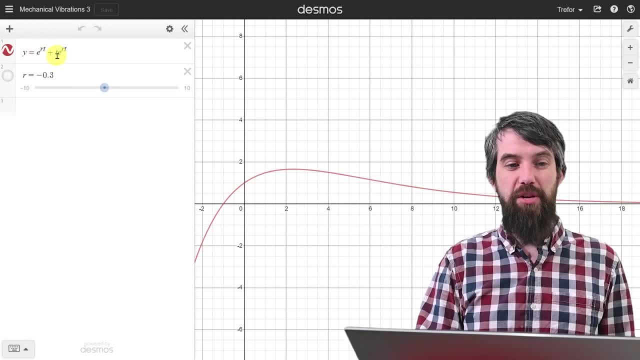 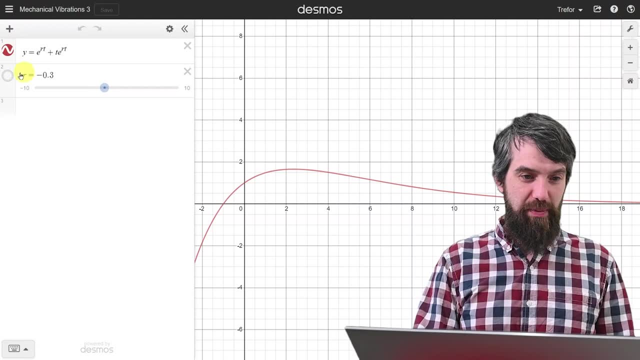 Graphing our critically damped case. I put in an e to the rt plus te to the rt. I just made my two coefficients both 1, just to illustrate the point. And what you see is that for this particular value of r, r does need to be equal to 0.. So what I'm going to do is I'm going 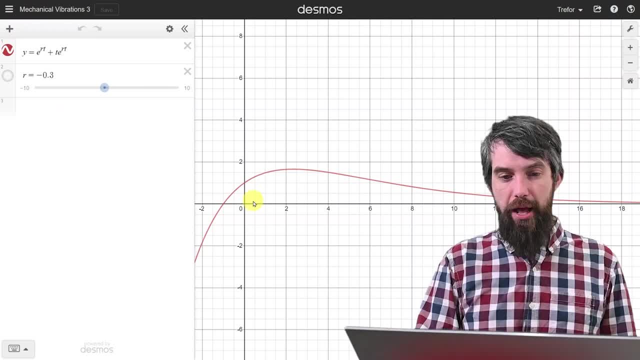 to put in an e to the rt plus t e to the rt. I just made my two coefficients both 1, just to illustrate the point. And what you see is that for this particular value of r, r does need to be negative, But what happens is when you start at t equal to 0, it increases. for. 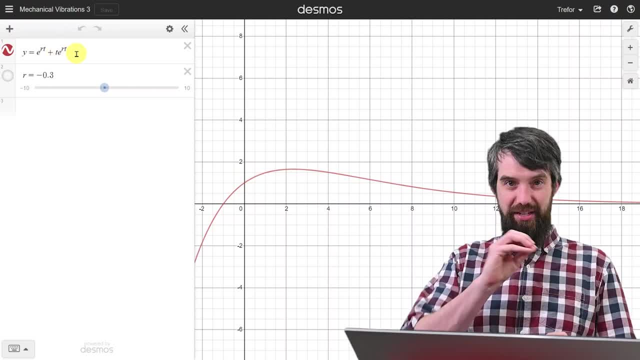 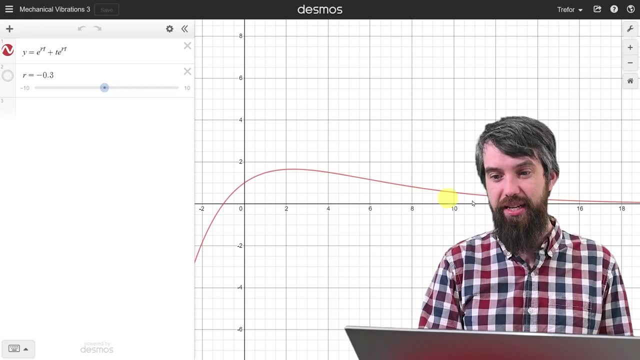 a little while, And that's because of that t term dominating. The t is causing this increase in the value. But then, as time goes on, it decays and decays, and decays, back down to the equilibrium position where, in this case, what we're calling y is equal to 0.. And indeed, 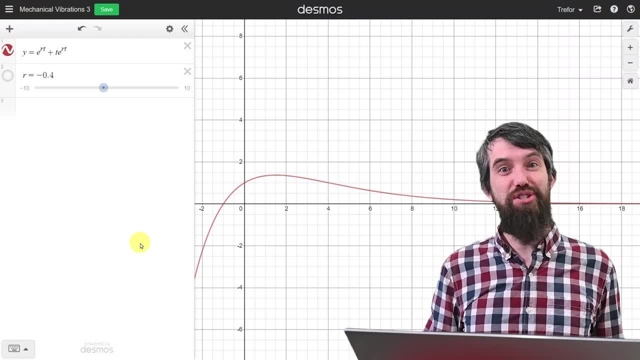 exactly the behavior you're going to get is going to depend on the initial conditions. I mean, I had sort of chosen initial conditions such that I would get 1 and 1.. And you can imagine one of those initial conditions could be about telling your initial. 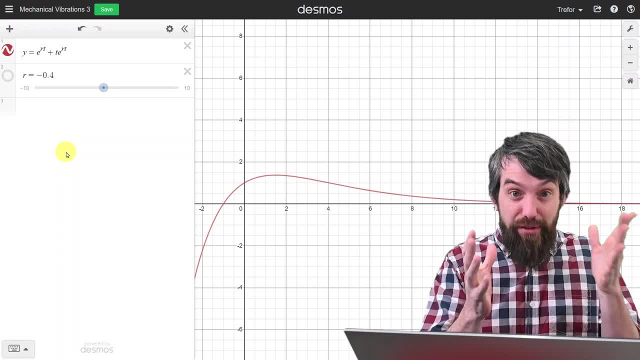 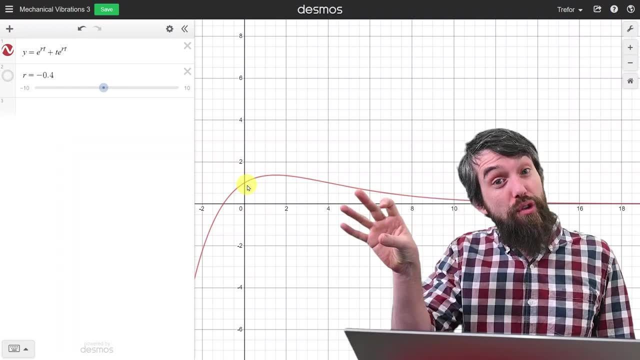 position and your initial velocity. So in this case, with this value of coefficient, from these initial conditions, what happens is that the displacement starts. if it's being offset a little bit, It goes further away. So perhaps that meant it had an initial velocity. 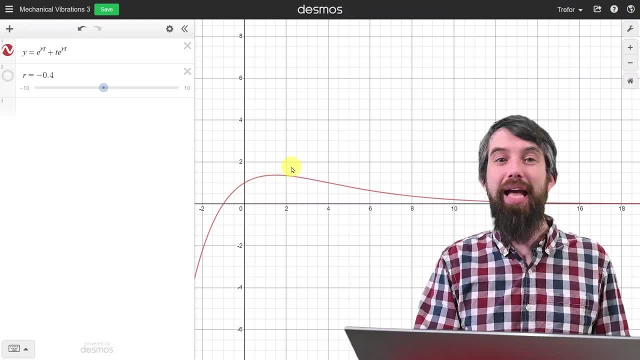 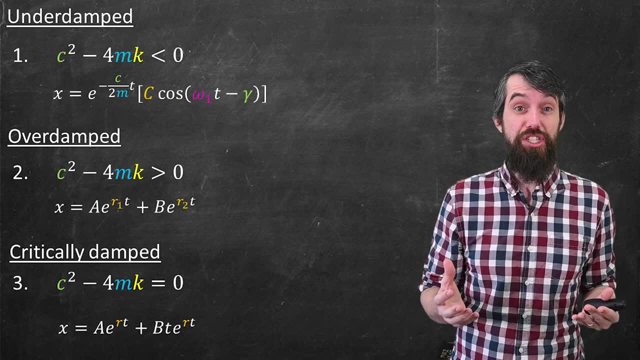 sending it to get larger And it goes away for a while And then it comes back And then eventually just comes in and settles right down at the origin. All right. So in the end the mechanical vibrations with friction can have these three different cases. The initial, 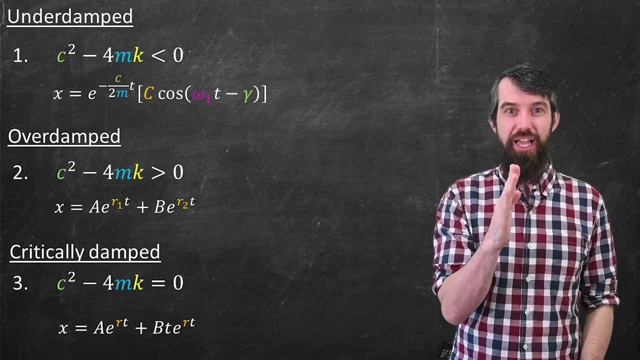 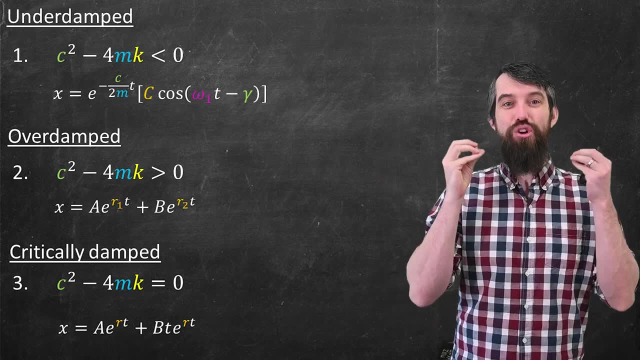 case, the underdamped case, where you do have these sort of nice oscillations. the overdamped case where it's just this exponential decay back to the equilibrium point and this kind of funky critically damped case. So if you enjoyed this video, please do give it a like. 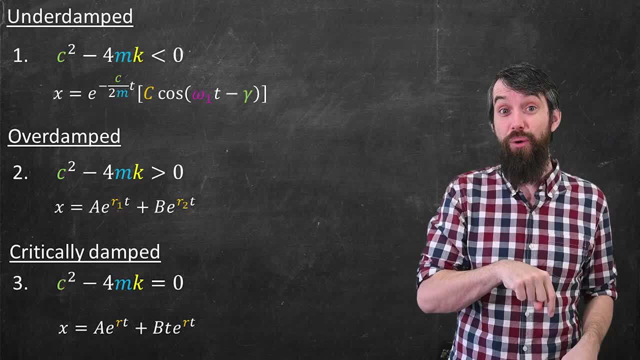 for the YouTube algorithm. If you've got any thoughts or questions, leave them down in the comments below And we'll do some more math in the next video. 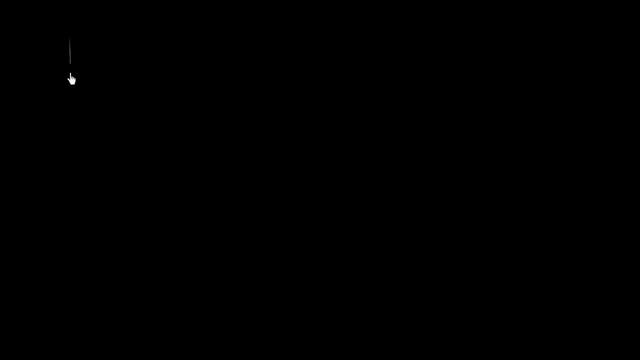 Let's say that we have a sheet of cardboard that is 20 inches by 30 inches. Let me draw the cardboard as neatly as I can So it might look something like that. So that is my sheet of cardboard And just to make sure we know the dimensions.